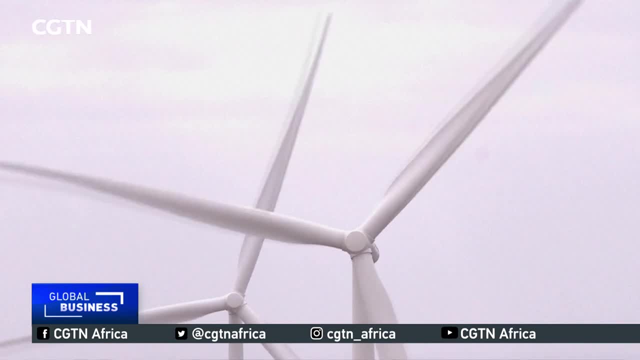 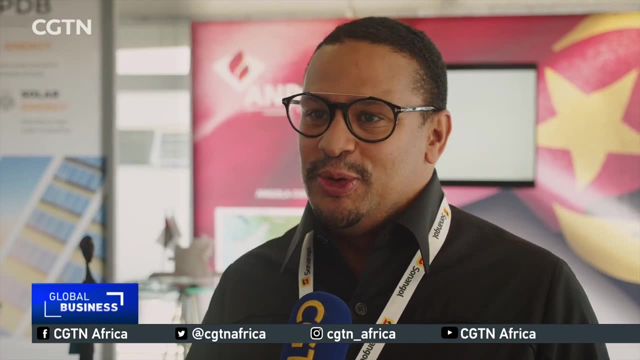 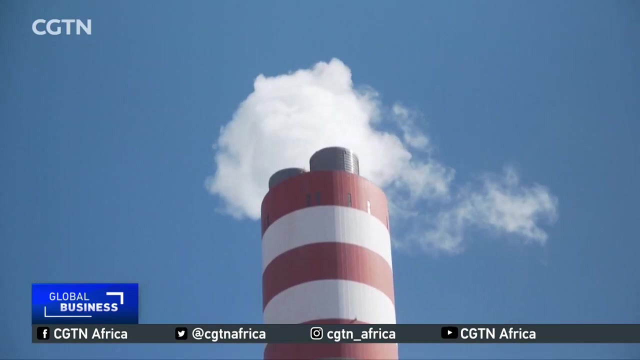 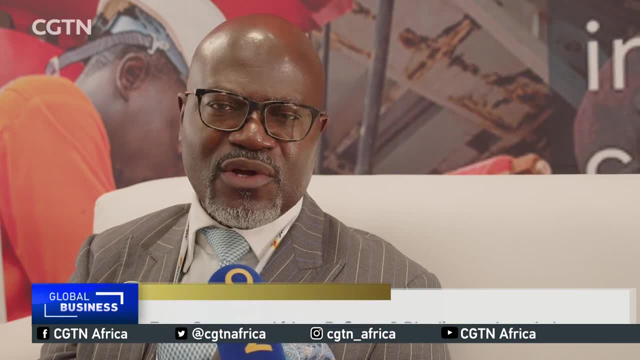 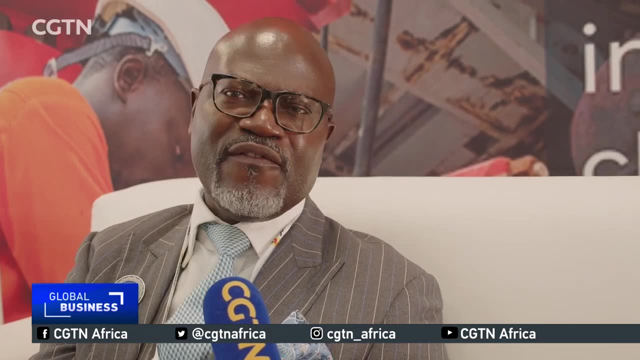 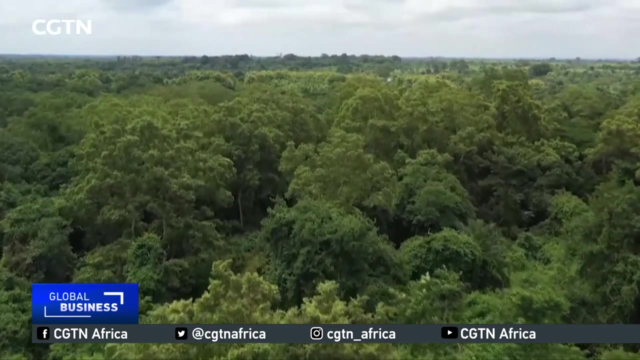 cumulative global CO2 emissions. to date, Africa has only contributed 2.73%, compared to 33% from Europe, 29% from North America, 29% from Asia. You cannot have the same rules, shall we say, for the 2.73% countries. As we go to COP27, there needs to be a discussion about how we 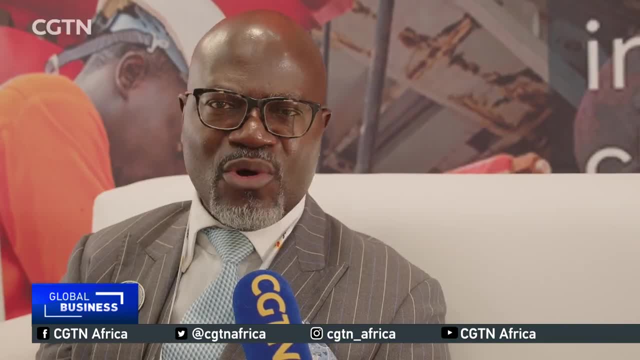 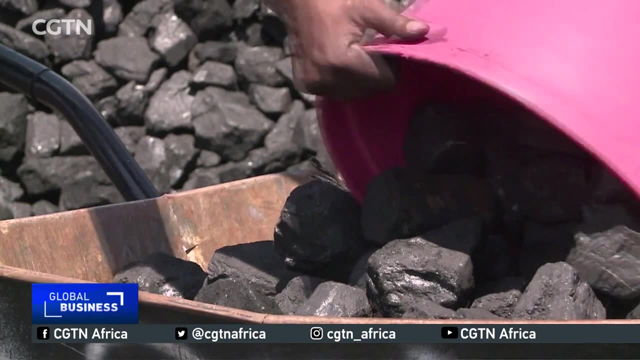 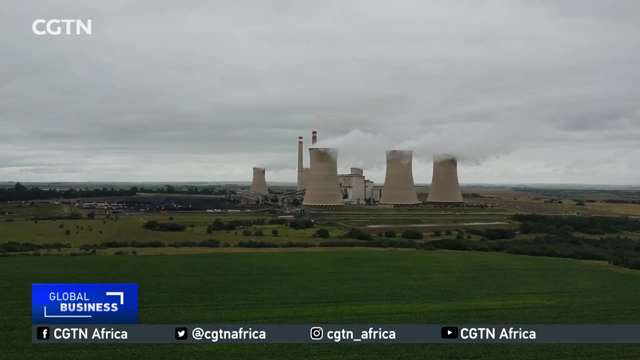 use what they call this climate budget such that it's allocated accordingly, so that the African countries can actually exploit their resources In a sustainable manner, but we should not be asked not to take advantage of our resources to empower our people. There's still a heavy dependence on fossil fuels across the continent. 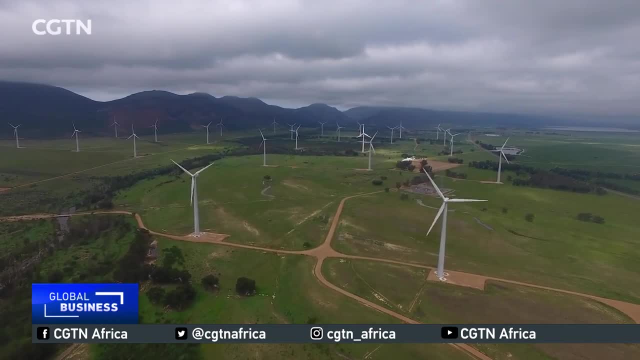 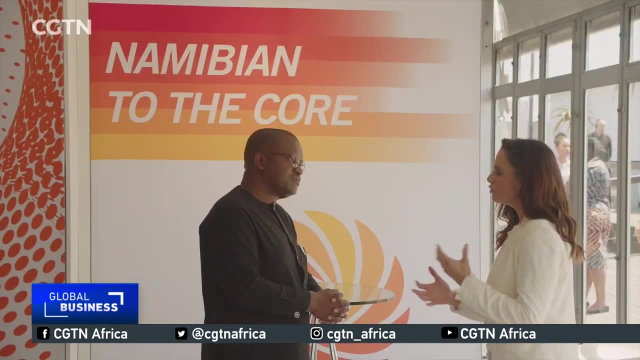 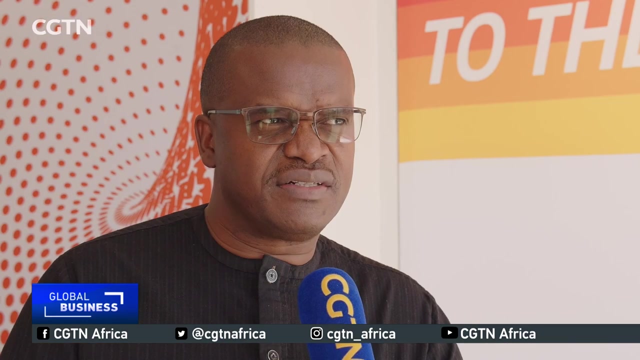 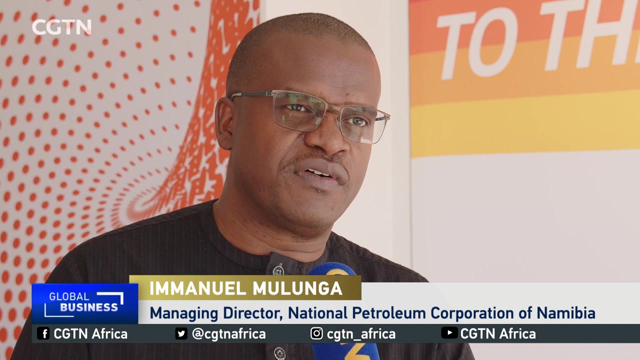 but many African nations are joining the global movement towards greener energy. Namibia, with its newfound oil and gas discoveries, is planning a comprehensive energy mix that could see the southern African country becoming a major energy player. Fortunately, green hydrogen and fossil fuels are not mutually exclusive. I mean one doesn't happen at the expense of 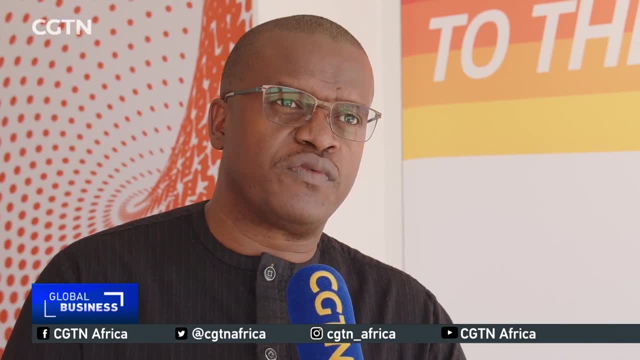 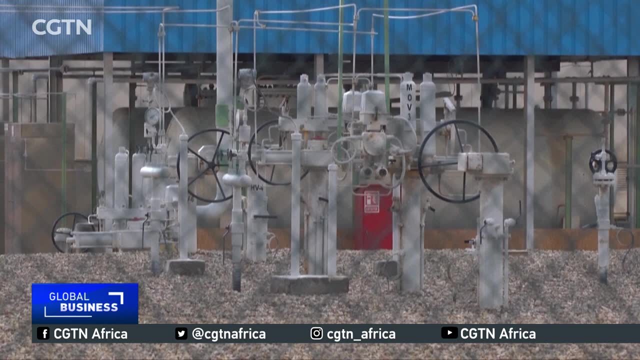 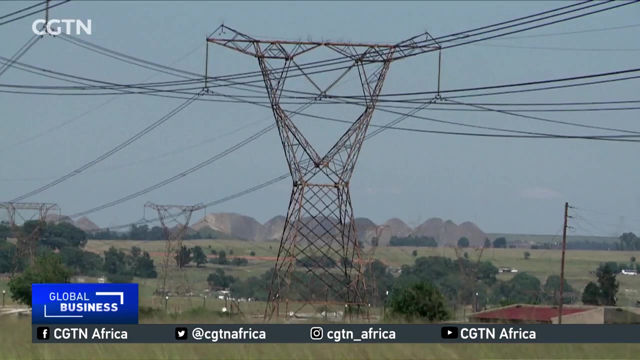 the other one. So we are going to forcefully go ahead to pursue the production of our discovered oil and gas because we believe it's all right. I think it's our time as Africans, with this green hydrogen potential that we have, we can combine green hydrogen with fossil fuels to make sure that. 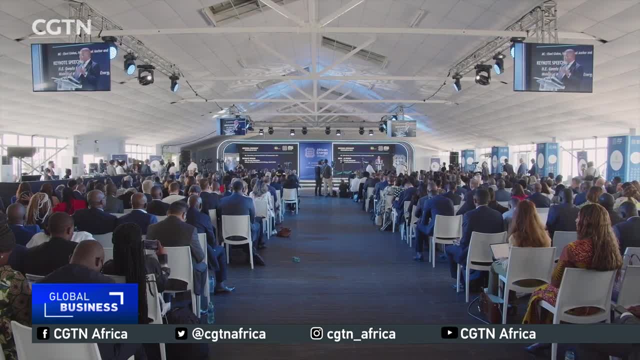 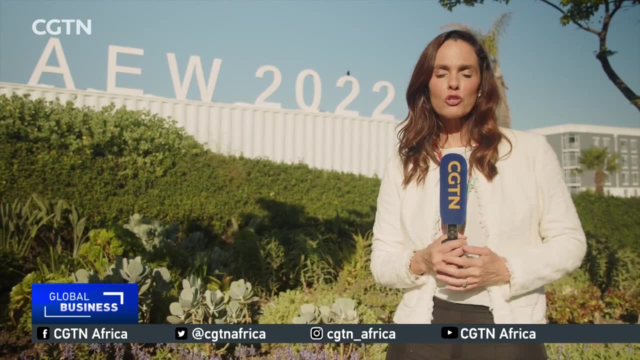 we make a huge contribution to the world. African countries rich in resources have the potential to change the continent's energy landscape, but they must work together to speed up the process towards achieving self-sufficiency. Julissara, Sijtjen, Cape Town, South Africa.